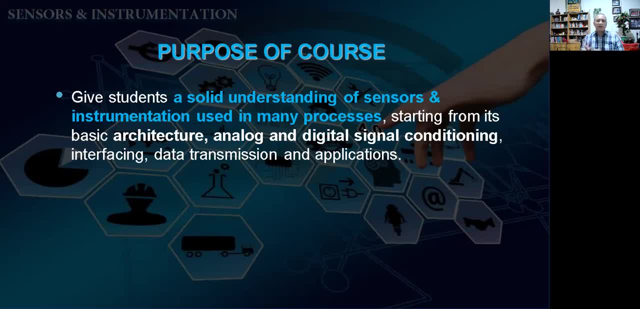 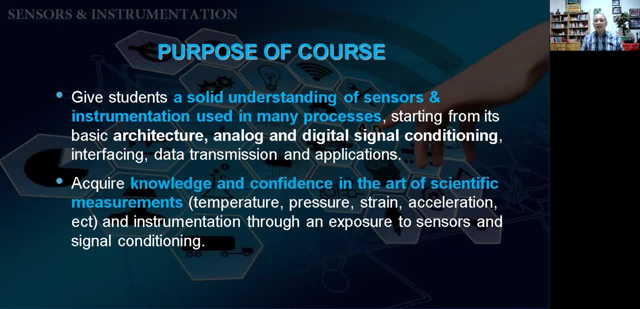 Controller or data acquisition system and transmission and application of that. And then, of course, the purpose is to acquire knowledge and confidence in the art of scientific measurement. Yeah, So how we actually measure all these physical quantities, you know physical entity, temperature, pressure, strain, acceleration, etc. And then how the instrumentation needed. 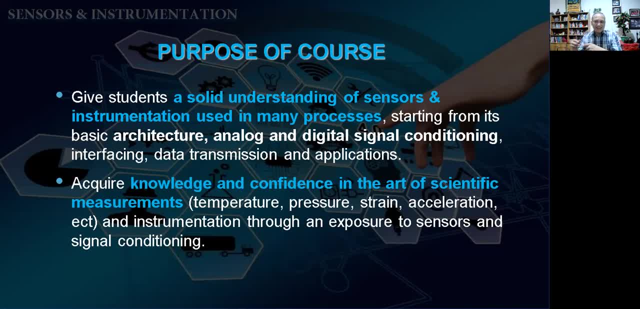 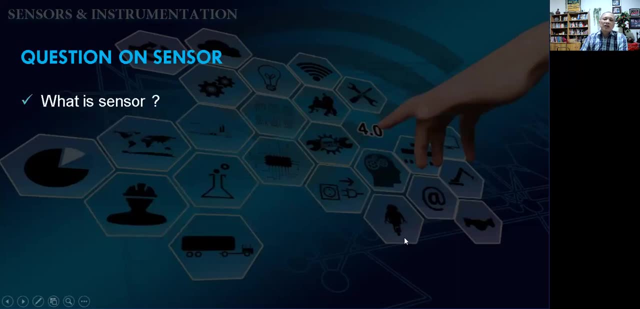 to actually to take the measurement, the physical measurement, and then transport it or transform it and then transmit it to where it is going to be processed further. Okay, So the question on sensor is: what is actually a sensor? We're going to discuss this and how a sensor works, Of course. 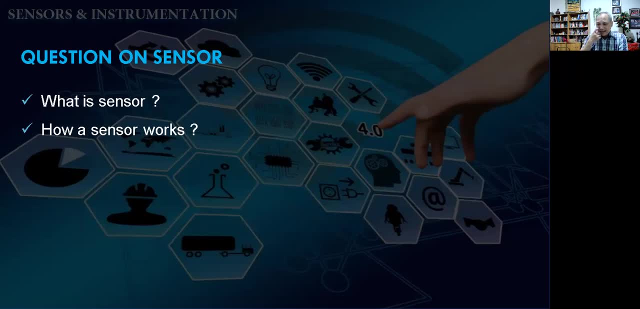 for different types of sensors it might work differently in principle, But of course, as a general principle principle, they are the same. Do our bodies have senses? of course, Otherwise we cannot really touch, feel, sense or taste. Yeah, Those are our senses. Why? 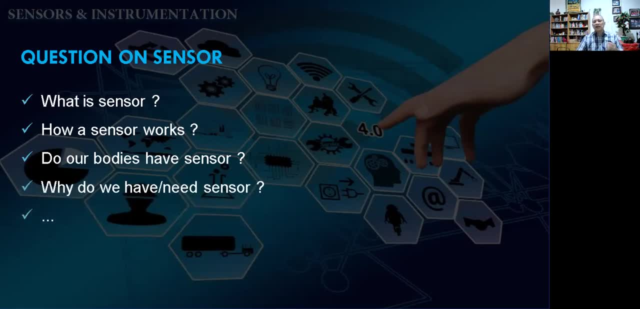 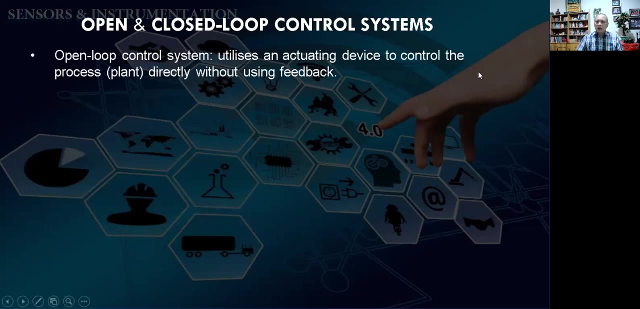 do we have or do we need sensors? We'll discuss this and hopefully this will give us, give you, a good foundation to study the needed topics in this course. Let's look at first the all open and closed loop control system. When we talk about open loop system, 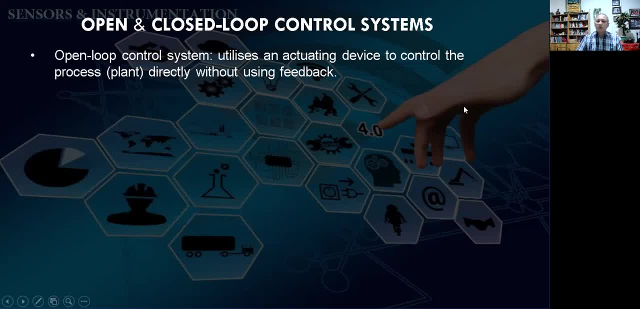 it utilizes an actuating device to control the process directly, without using feedback. So there is no feedback to the brain, There is no feedback to the controller of what happens in the system. So it looks like this: So we give the input and then the actuators. 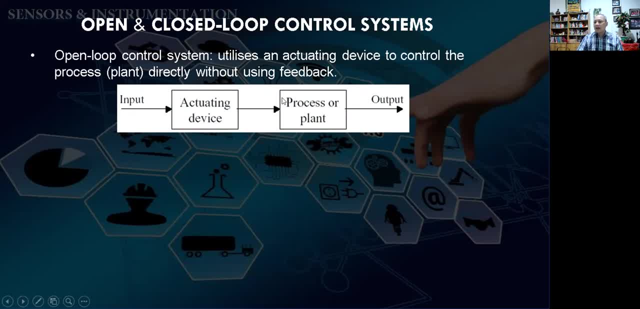 and we'll do something to the process or plant and then it will give an output. Of course, whatever the output is, it's not being fed back to the input so that to be measured or to be made better or to be improved or so on. 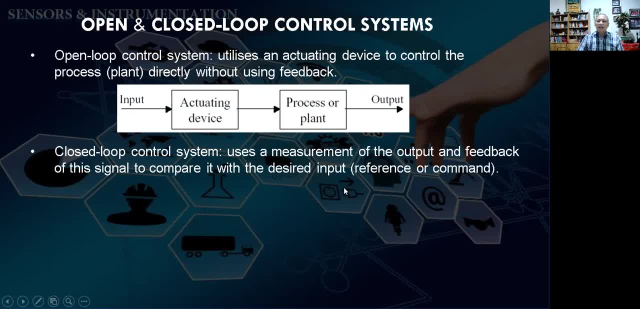 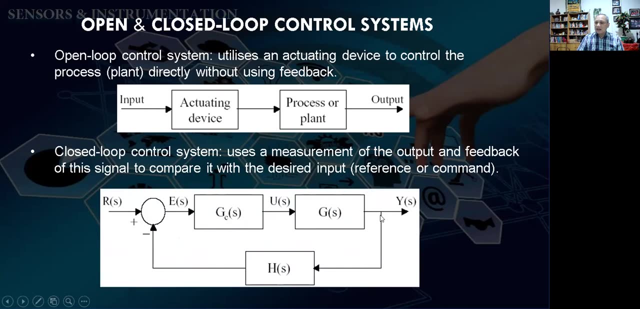 But on the other hand, if we have closed loop control system, the difference with the open loop control system is that the signal, the output signal, is being compared with the input, the desired input. So it looks like this: So there is this HS that will tell the brain. 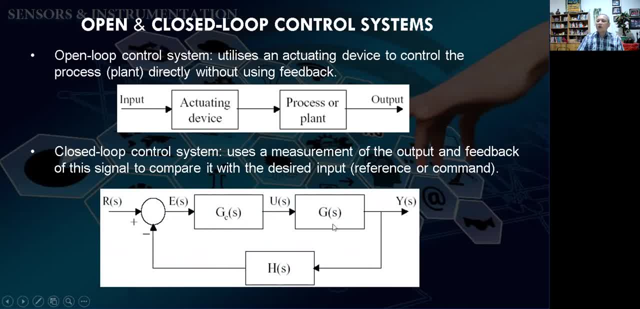 or the input, or compared to the input, what is the situation, the condition, the state of the output? And how do we do that? And we do it by sensing it. If it is talking about position, then this is a position sensor. 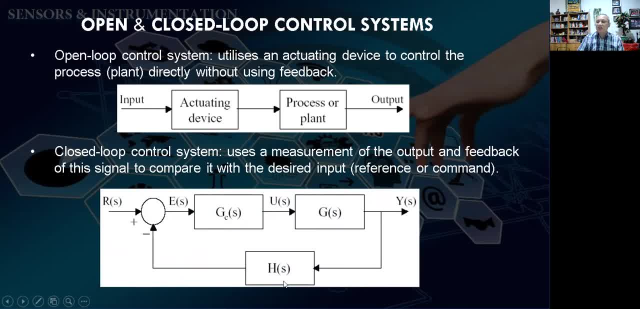 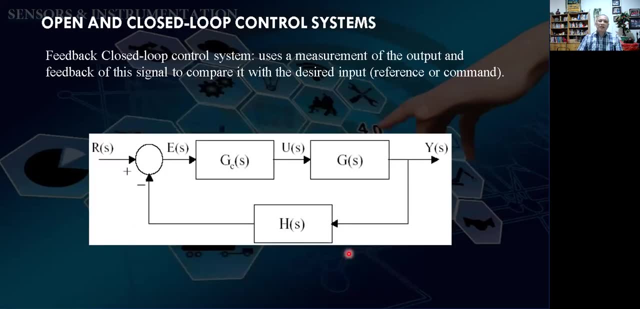 If it is about pressure, this is a pressure sensor. So this is this H thing. Let me put my laser pointer here. So this HS is essential. That's how it fits into a closed loop control system. So if we look at it bigger, a bit bigger on that. 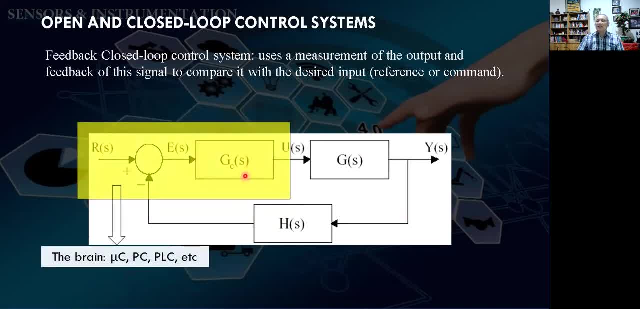 actually, when you see it, the GC here is the controller, whatever the controller you like to apply- And GS is the plant And Y is the output, HS is the sensor. So the sensor is being fed back to the input being compared to the desired input here. 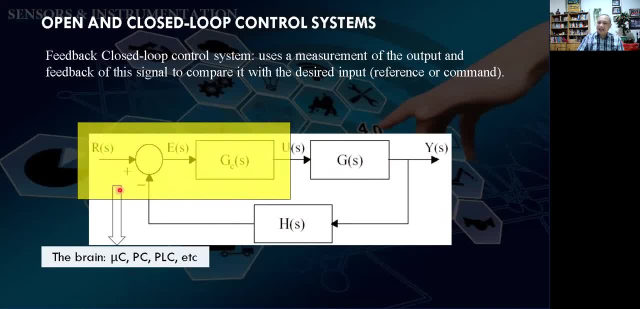 Now, this yellow shaded box is actually the brain. It can be microcontroller, PC, PLC, whatever it may be. So this is the brain. So the sensor output will be received by the brain and then compared with the desired input, And then it energizes or it controls the controller here. 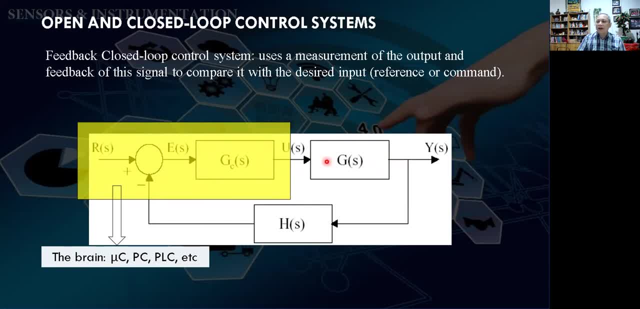 to give output, And then the brain is then put control to the plant, and so on and so on. So this is how that sensor play a role in a closed loop control system. So what is sensor? Sensor is a device that receive and respond to a signal. 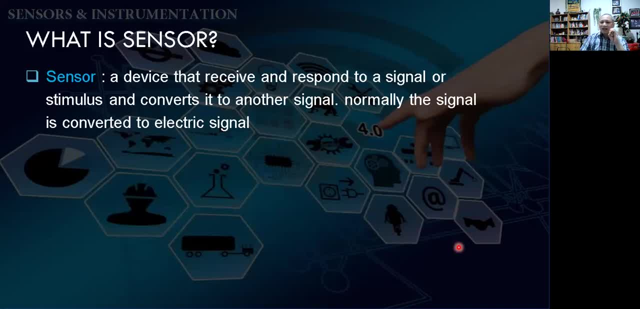 or stimulus and converts it to another signal. Yeah, that's normally. the signal is converted to electrical signal. Now I would like to just mention the difference between sensor and transducer. So in this course I will just call it sensor. That's the name of our, the title of the course: yeah, 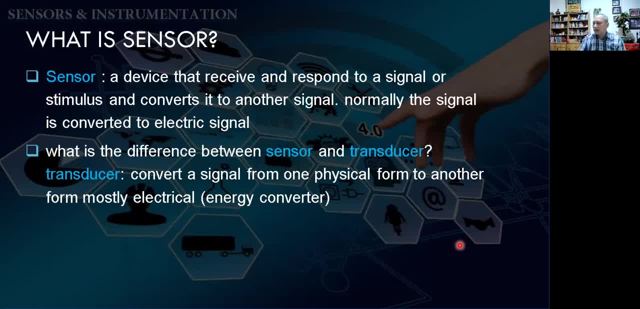 Sensors and Instrumentation. It doesn't mean that we are not talking about transducer, but transducer. what is the difference between transducer and sensor? Transducer is actually every sensor is a transducer, they said, but not every transducer are sensors. 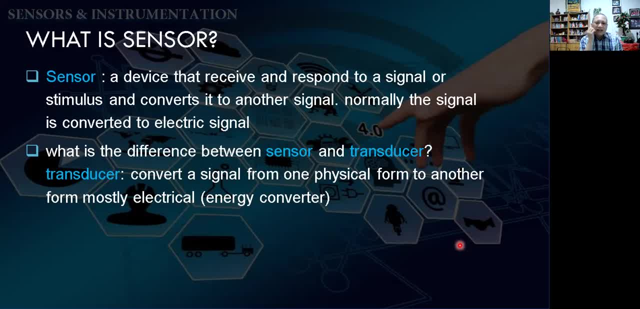 So transducer, basically, is more like an active sensor, So it is like a conversion or transformation of energy from one form to another. Usually this is when we're talking about. let's say, we measure a position, we measure a pressure, we measure some kind of physical quantity. 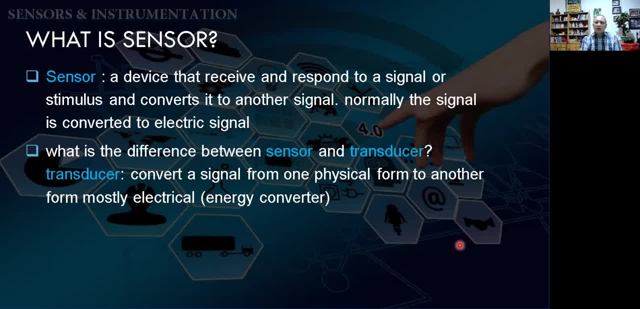 and then a transducer sensor will somehow change something. For example, if you have a transducer sensor, for example, if you have a transducer sensor, for example, a resistant temperature detector, So if the temperature change, then the resistance value of that sensor will change. yeah, 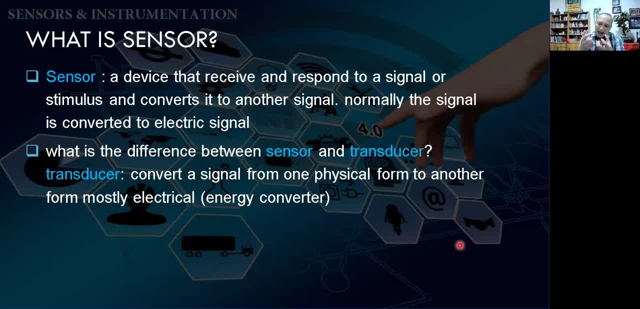 That is a sensor. But if this sensor then will be transforming its signal from that physical resistance value and then compare it to, let's say, a voltage value to be fed back to the controller or to the PC, then somehow we can call it a transducer. yeah, 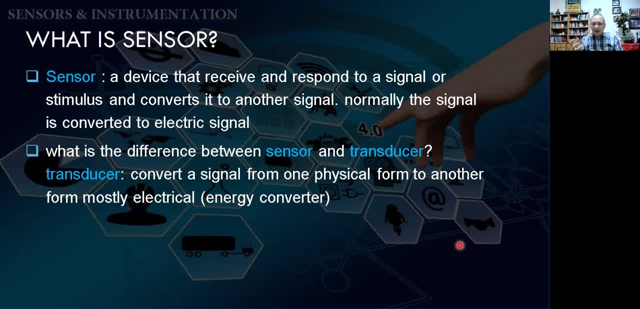 So the conversion to another quantity, to another entity. it makes it transducer, but it doesn't matter. All along this course, I will call it sensors, yeah So, just for the easiness of mentioning it. So, but there is another one: sensor versus actuator. 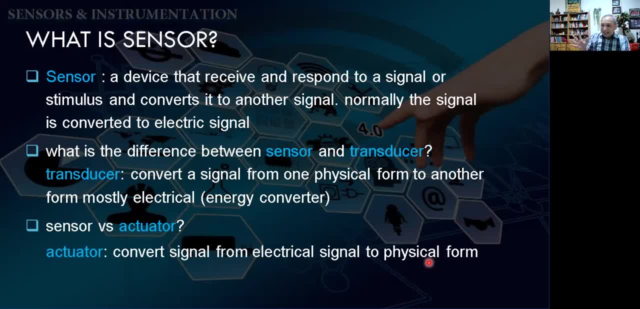 So there is another one, sensor versus actuator. Our sensors are actually the opposite: The conversion of the energy conversion, the boss person, energy conversion, the other way around. So if a sensor is converting signal from physical form to electrical form, then this one is the other way around. 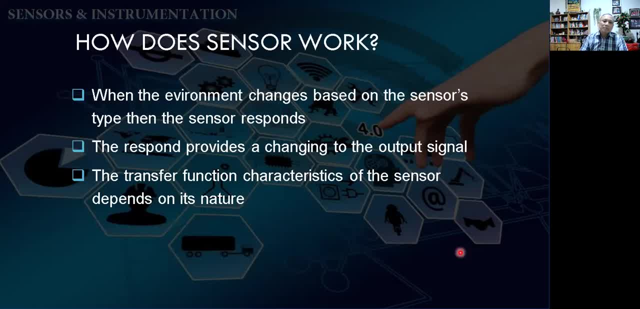 which is electrical signal to physical form. okay, Just a definition. Yeah, Okay, Okay, Okay Okay. How does a sensor work? environment changes. this is how generally sensor works. so when the environment changes, based on the sensor's type, then the sensor response could be: uh, the, the the charge in pizza, electric piezo. 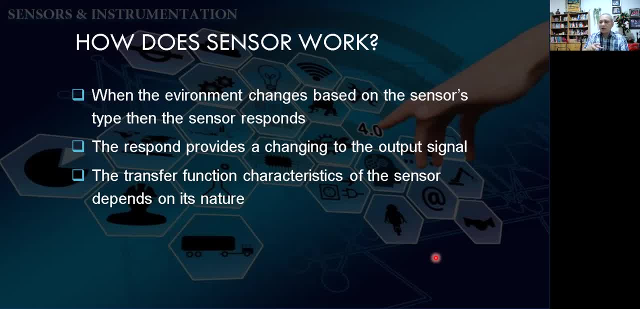 electric uh can be changed, or in temperature resistant detector, the temperature. the temperature will change the, the value of the resistance. similarly, when we're talking about um, pressure sensor, things like that, yeah, so then there is, then the response provides a changing to the output signal if we are connecting it to a circuit. 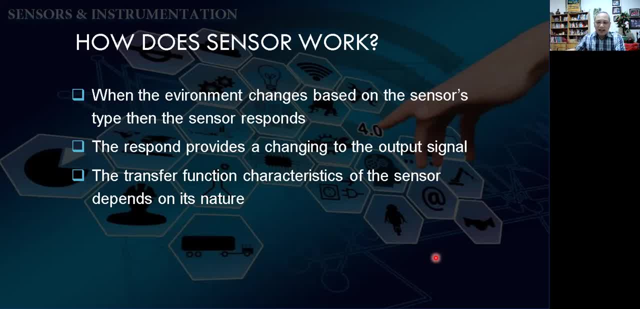 like a wisdom bridge, and then it will give a different output and then the transfer function characteristic of the sensor depends on its nature, of course. yeah, so that's how it works. so the physical uh changes will change a physical uh uh quantity or characteristic of the sensor. 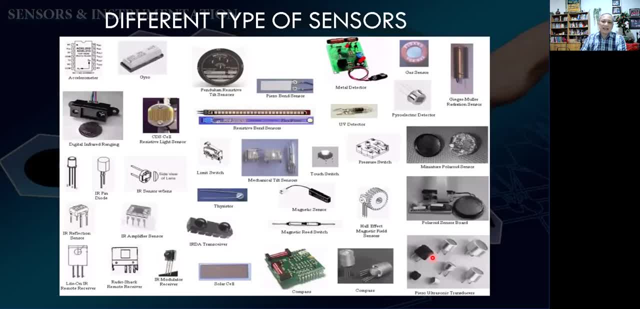 that's how it goes, and then we transform it to another signal. so this is different type of sensor. you can look at it. uh, quite a view, there's a pizza band sensors. you know, when you're bending something by pressure, then the value change. uh, pyroelectric and what else? magnetic sensors. 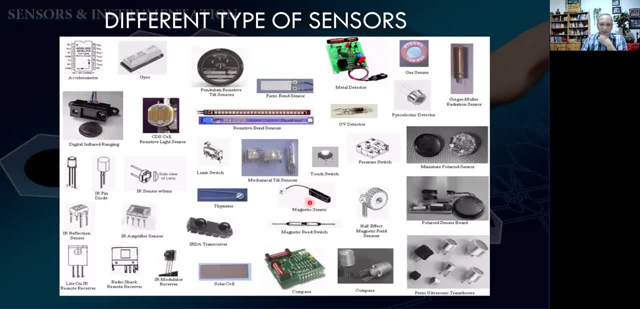 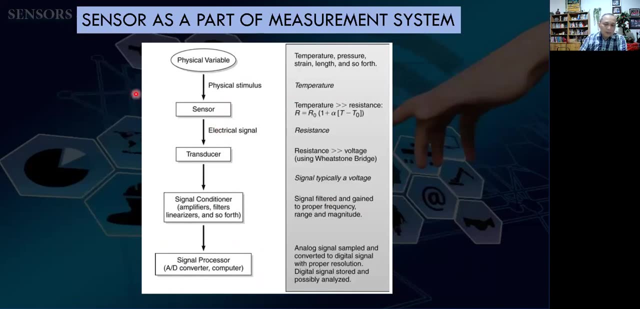 we have the proximity sensors- yeah, because we can check whether it is uh made of uh metals or not, and so on. there are so many of these. you can also google it easily, yeah. and then, of course, the sensor is a part of measurement system, so it's always a part of measurement system. it's part of process control system. it's part of a 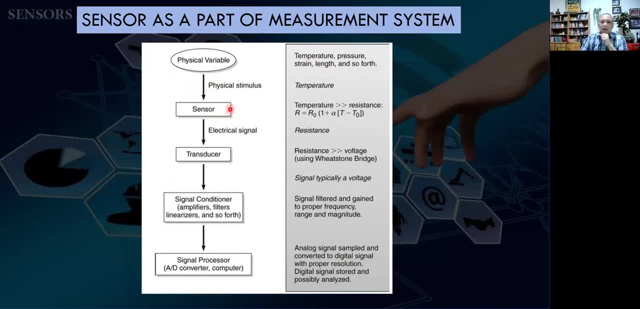 bigger system. yeah, so when physical, physical variable and then it is changing some uh stimulate some uh physical quantity in the sensor, then the sensor, when we call it before a transducer, so we change it to electrical signal. and then this electrical signal somehow we need to condition it so that we can measure whether we filter it, uh, to avoid to get. 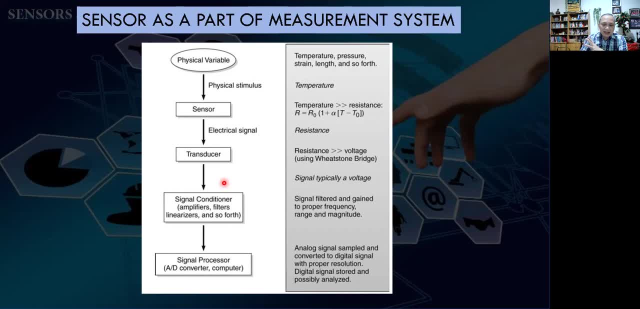 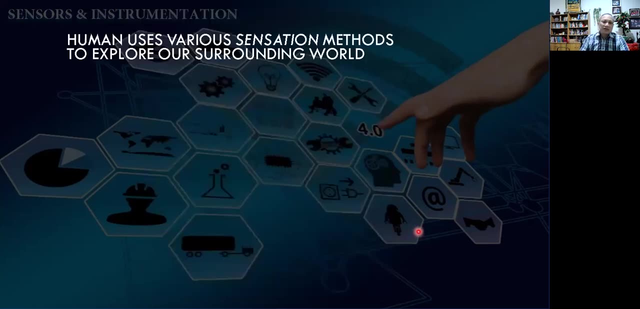 rid of any noises, uh, any unnecessary uh signals, and then we can amplify it, linearize it and so on and so on, and then we can process it afterwards. this is talking about analog to digital uh converter. yeah, okay, so as part of system, so human uses various sensation methods to export our surrounding world. this is. 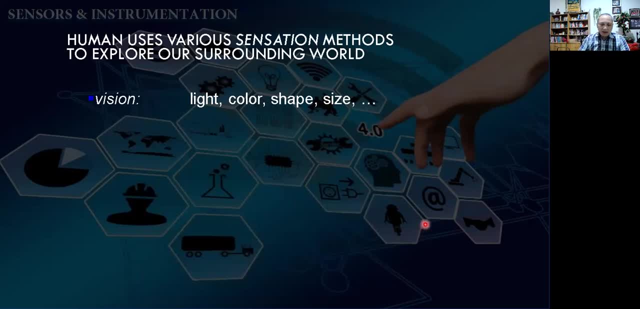 just a quick uh cover on our sensing, yeah, our senses, a vision, sound, yeah, light, vision, color, color, shape, sound, the tone, the volume, the frequency, things like that. so, uh, a smell, odor, taste, what else, touch, smooth, rough, feeling, hot, cold and motion and all that, so this actually can, can be the basis of our 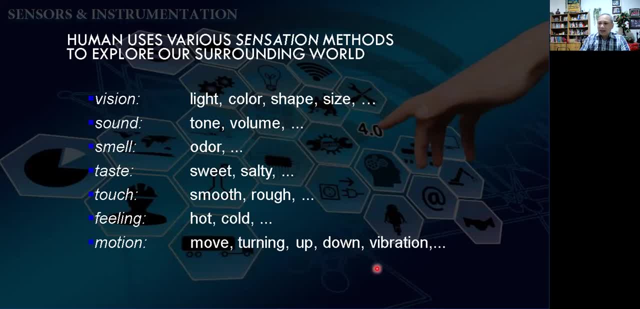 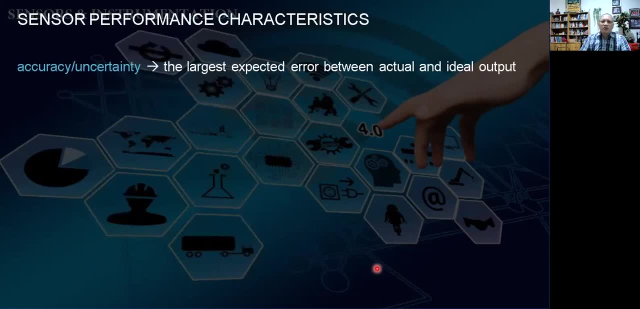 sensing mechanism in the engineering world as well. yeah, okay, so sensor performance can also be classified to certain characteristics. so accuracy, you know, you know. uncertainty is talking about the largest expected error between actual and ideal output. so you, you should, we should, as engineer, we should know this term, you know. uh, when we are measuring something, what is the question next? 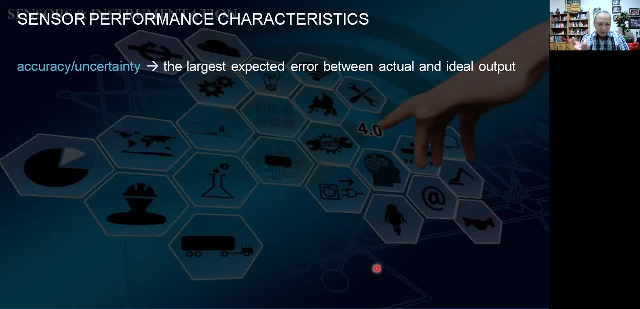 question is: what is the accuracy of that value that you're measuring? is it reliable? you know, if the accuracy is not, it's not so uh, so small. if the accuracy is not so good, then probably the whole measurement could be just uh, bias this discrimination resolution. so a minimum detectable signal fluctuation. the resolution of your. 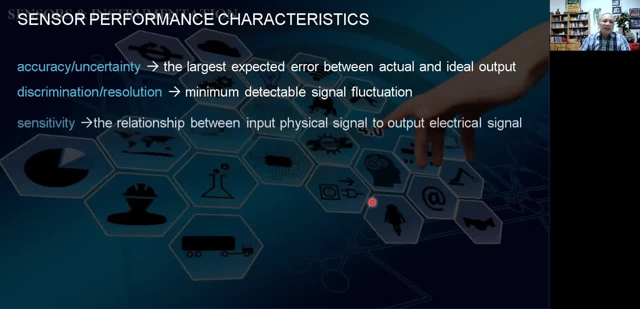 laptop. the resolution of your measurement is also very important. sensitivity: what about the relationship about your input and the output if you change the output, uh, a lot, but the input a lot, but the output is just changing a little bit. probably it's not very sensitive, so that should. 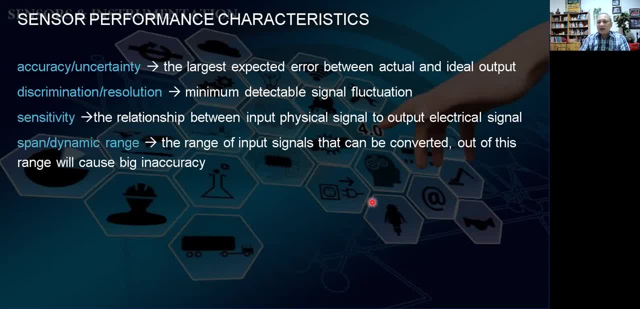 be also in uh, taken into consideration: span and dynamic range. the range of your measurement, uh uh. does it cover the needed uh measurement or not? yeah, linearity, you know there is a deviation in every every measurement that we do. if it is not so linear then probably we cannot really come up to a. 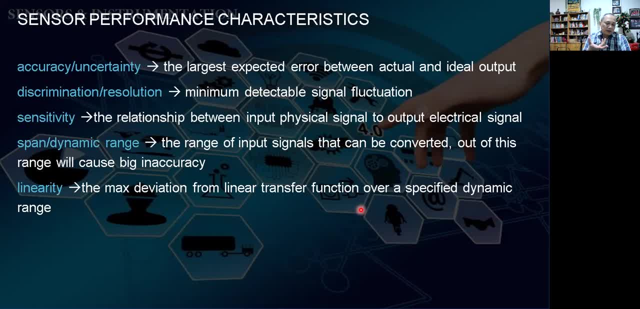 good conclusion or a straight conclusion saying that possibly we want to say that if you keep increasing the input, the output will be increased. well, for non-linearity probably is not the case, so linearity is also must be taken into consideration. hysteresis, right. so anyway, now there's even more data about the. 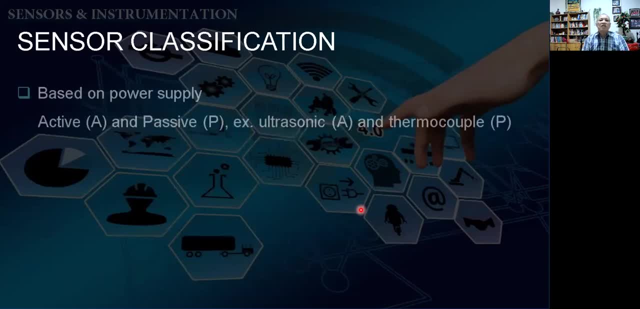 yeah, oh, oh. yeah. So sensor classification, sometimes we call it based on power supply, active and passive. So active, like ultrasonic, it means that it is active because it keeps sending signal And then when there is changes in the receiver, so transmit. 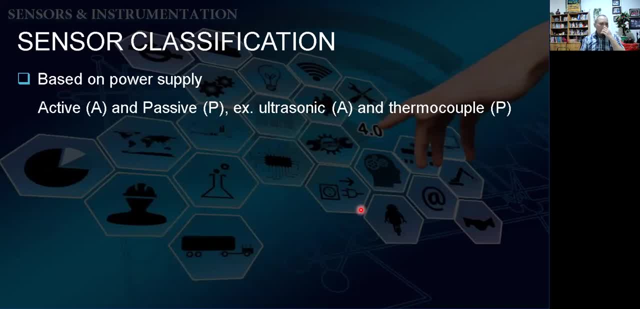 and then will receive. Like, for example, ultrasonic wants to know what is the distance of an object, So it keeps sending signal, So when there is something passing before the transmitter, and then it will be reflected back, then it can measure, it can sense that there is some object. 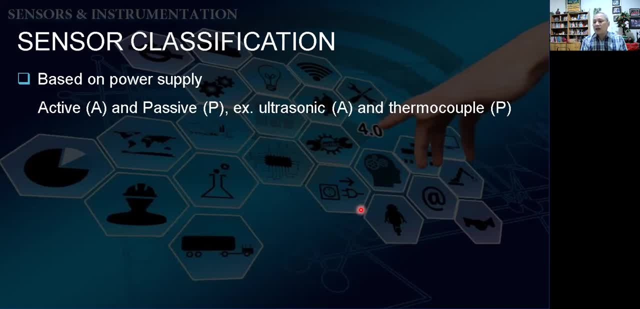 on the way, in the way. So it means active, But thermocouple passive sensors are sensors that are not really active, of course, in a way that it doesn't trigger the measurement, It doesn't trigger the process, It's just. 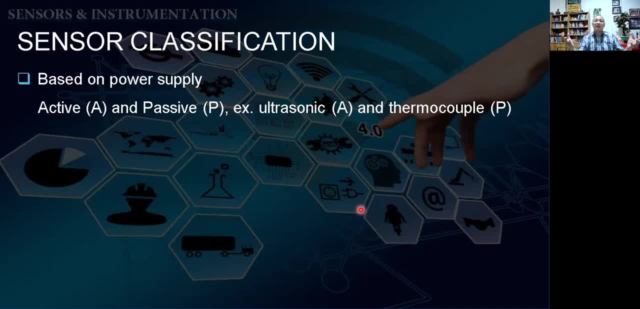 Waiting thermocouple, waiting for the temperature to increase, And then the thermocouple will be having some changes. Then that's when the sensor is sensing something Based on the nature of the output signal. of course you know it: digital signal, analog signal, like encoder. 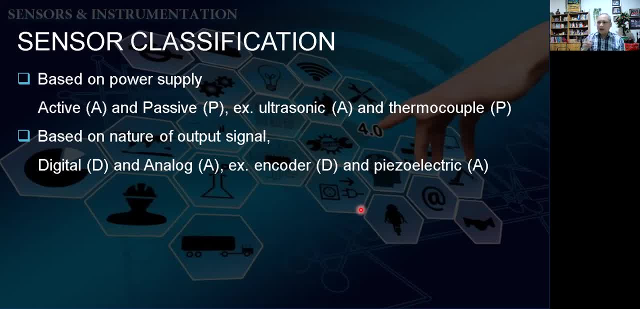 Encoder. when we are measuring a rotation of something using infrared, for example, then it will just say: on and off, on and off, things like that. But piezoelectric is active. It's analog because whatever the pressure that you put on the ceramic or on the sensor material, 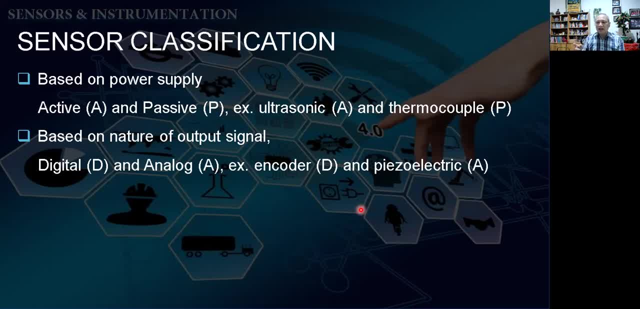 then it will give a real number, output things like that. So it is analog. And then, finally, based on the operational mode, there are two: deflection by deflection by null mode. Null mode is you have to reset it to, let's say, null or zero. 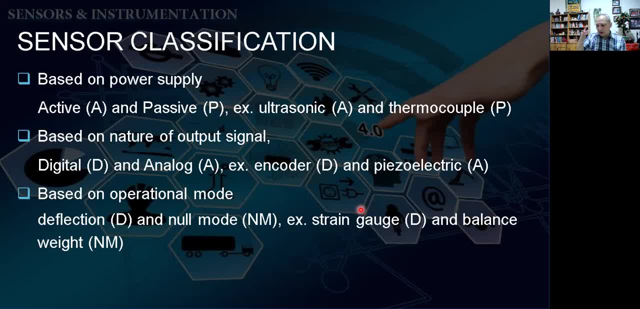 like a balance weight. If you measure it When it is not null mode, then at the null mode state, then it is not valid, While strain gauge is based by deflection, Let's say it is whatever the state is. That is the normal measurement, the normal value. 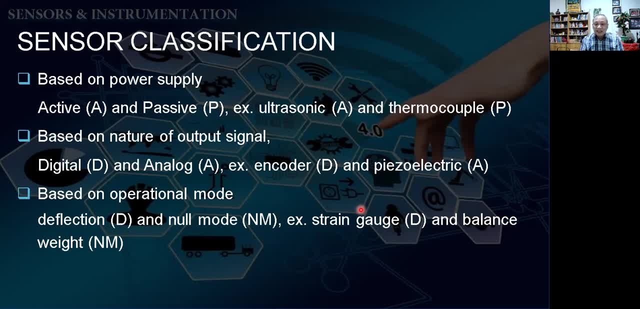 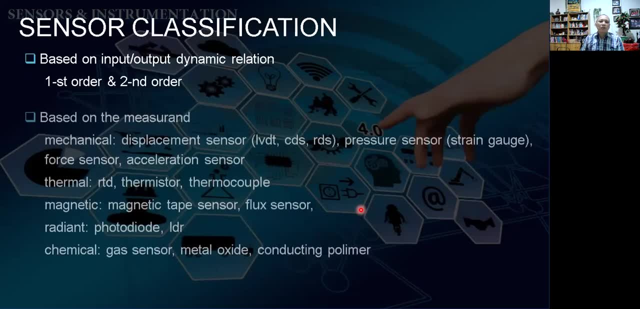 So when we are measuring something and it deflect, then we know it is having a certain value from that deflection. OK. So classification: OK, I would say based on input and output dynamic relation. there are first order system and second order system. 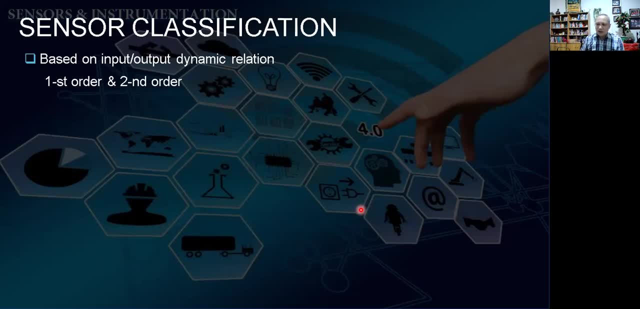 We're just discussing. even in the previous semester maybe you studied the system: response of components, response in transfer, function, I would say, when given a certain input. So what will be the behavior? So the behavior. of course, there are third order, fourth order, 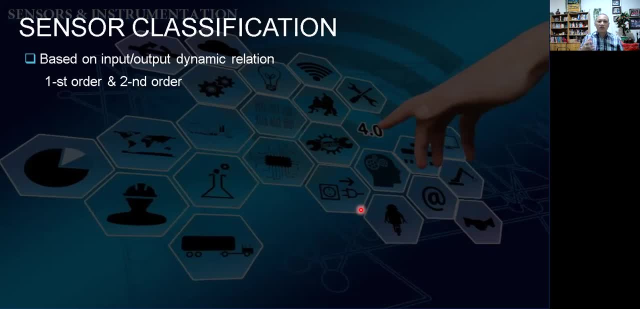 Usually we are simplifying it to first order and second order, because higher order usually can be simplified, I would say to first order and second order, even though it's not that easy, but because the constraint of this study is not within the higher order. 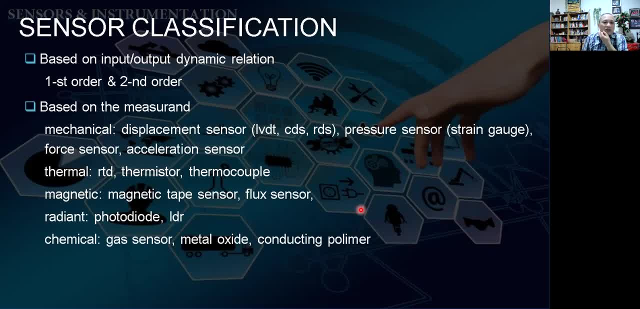 So we're just focusing on the first order and second order, And then based on the measurand. so we're talking about mechanical, which is displacement sensor, LVDT, compact displacement sensor or reflective RDS displacement sensor, pressure sensor, strain gauge. 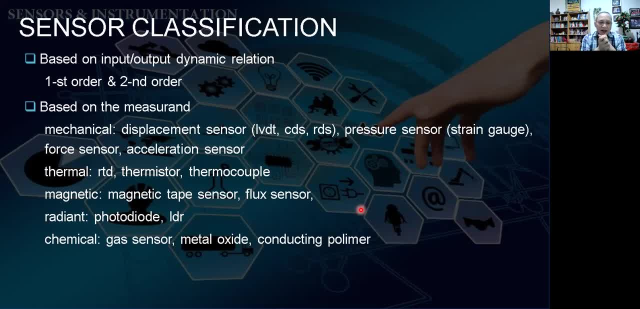 force sensor, acceleration sensor, thermal RTD- I was mentioning resistance- temperature detector, thermistor, thermocouple, magnetic radiant photodiode- this is like a ray- And then chemical gas sensors And then based on physical measurement variables. 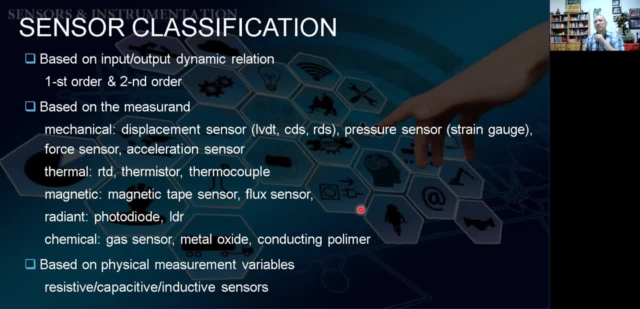 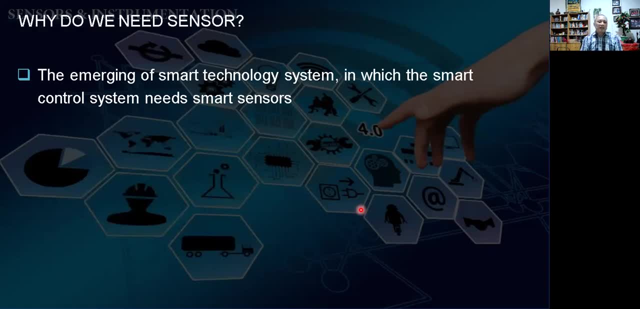 so how it varies, like resistive, capacitive, inductive sensor. So these are the sensor classification. Why do we need sensor? Of course, the emerging of smart technology, Everything needs sensor because we want to respond to a certain state. 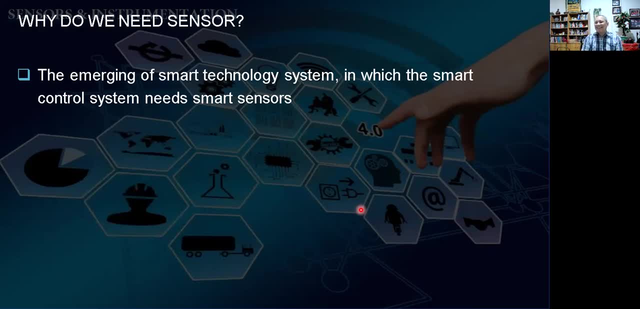 So smart, for the system needs smart sensors, Otherwise I'm going to be smart if my input is not smart. And secondly, using sensor in relation with the control system, it increases the efficiency and effectivity. So, like our air conditioning home. 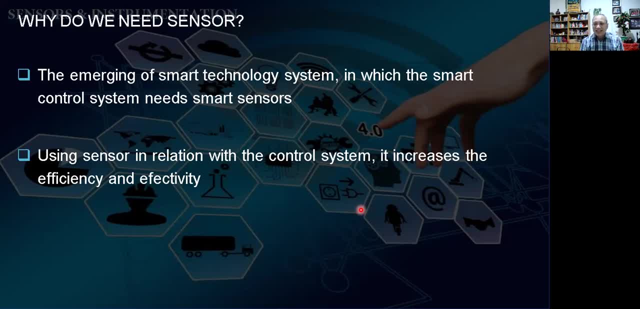 So it has sensor. So when we want it to be in 20 degrees, so it will try to reach 20 degrees Celsius temperature, but it will stop as soon as the compressor will stop as soon as it is reaching 20 degrees. 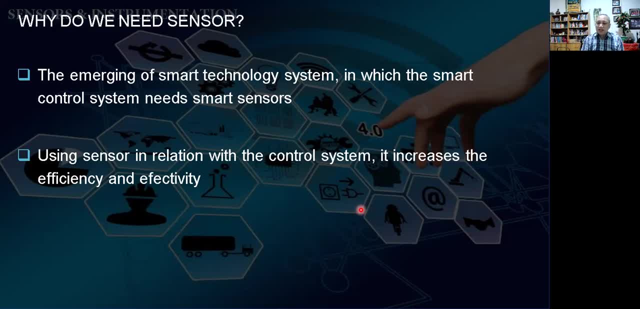 So then the compressor will stop. Yeah, Yeah, It will stop for a while. Yeah, So it means that it is reducing the usage of the fuel or the electricity, And sensor technology can be used as data logging in real time and long distance monitoring, of course, 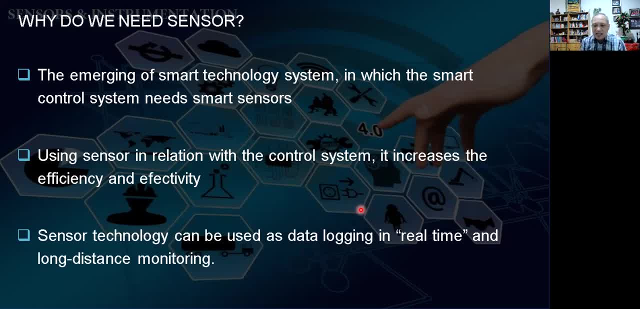 When we can put it, especially in the Internet of Things this day, IOT, then we can put our sensors and then we can log the data in real time and then we can also monitor it from a distance. So it's magnificent these days, yeah. 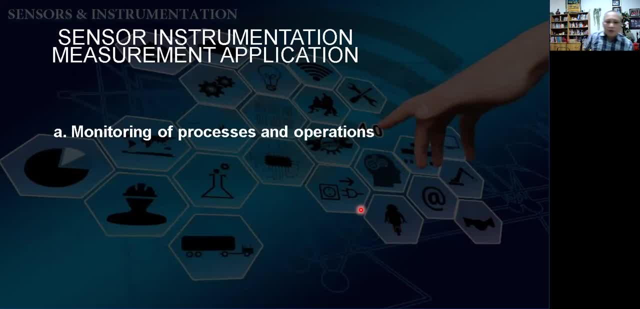 And application. Yeah, Now there are three here: Application for measurement, instrumentation, monitoring of processes and operations. Secondly, control processes and operations. So we monitor and then we control it And then we are doing experimental engineering analysis in the lab. 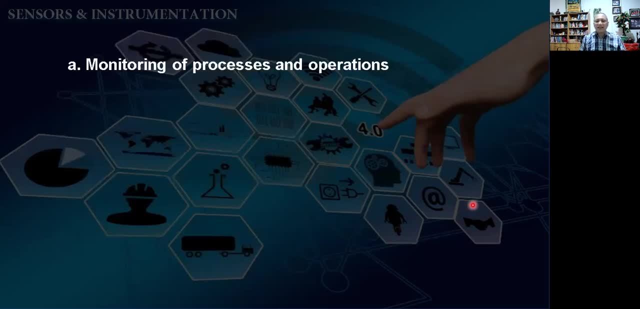 So what we can do about it, what we can improve things like that. Yeah, First, monitoring of processes and operations. So this is referring to situation where the device is being used to keep track of some quantity Mm-hmm. 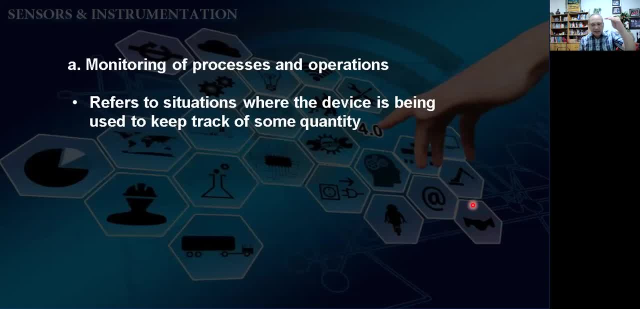 So we may not monitor it, So we want it to be at this certain level, Then in that case we need to keep tracking it, So otherwise we are losing point or target. Simply indicate the condition of the environment. Yeah, what are the condition of environment? 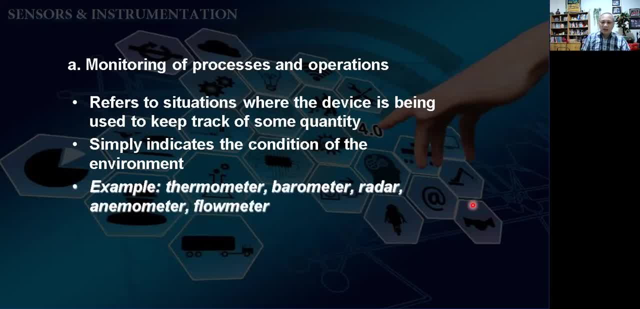 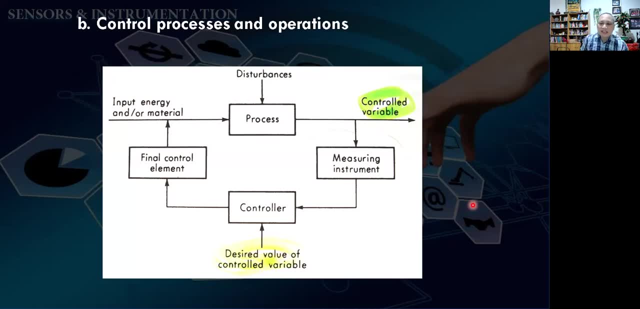 An example: thermometer, barometer, radar, anemometer and flow meter. This is also an input so that we can make a decision. And second, about control processes and operation. This is looking like the block diagram of a system process operations. 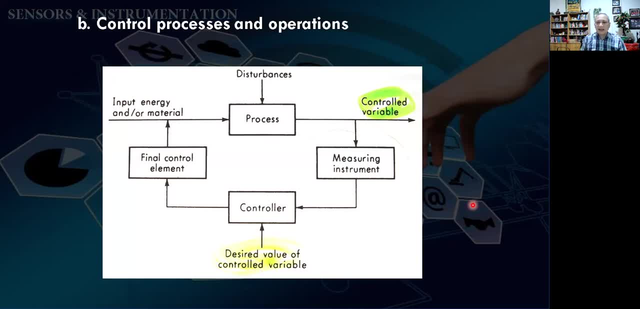 So there is input to the process, There are also disturbances, and then it outcome, the control variable, And then we measure using sensor measuring instrument And then also in that, and then we put back. this is similar to my block diagram before. 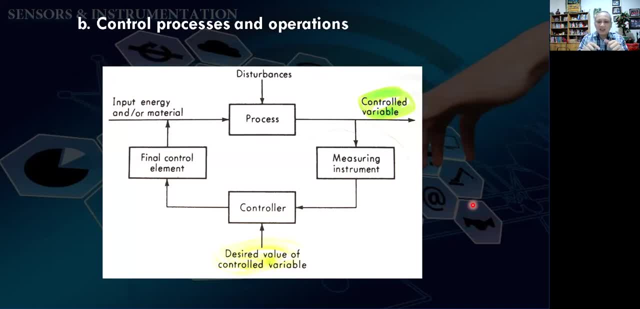 but the shape, the orientation is a bit different, but actually it is the same, The sensor being fed back to the controller and the controller also will compare the desired value and the real value and then gives to a final control element so that it can do something with the process also. yeah, 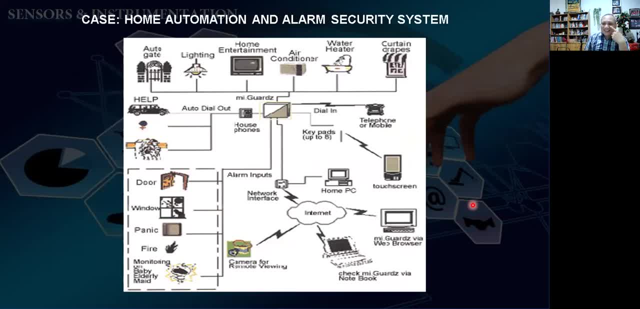 And then this is like a home automation, If you look at this, how one certain point can control or monitor many things. yeah, It can control the auto gate, gate of the house, lightings, home entertainment. You can just turn it off and turn it on. 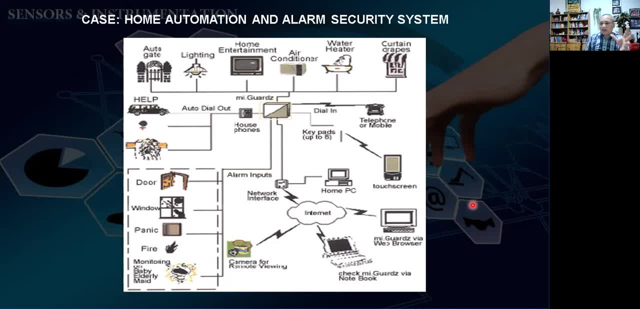 through this connection, whether it is local alien network or whether it is controlled by internet. yeah, Along a distance, control Water heater, curtain, things like that. Everything, yeah Everything can be connected to internet. look at that, So we can even look at the CCTV. 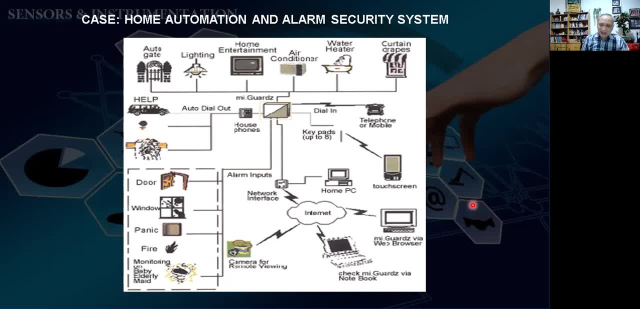 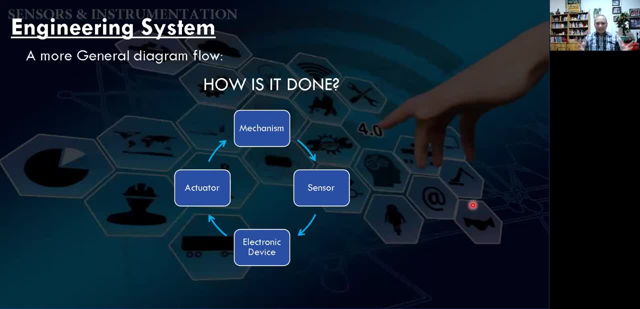 and so on and so on. So this is just an example picture I took from the internet. Okay, the engineering system, a more general diagram for how is it done? So, when you look at this, this is mechanism, system and then sensor actuators and electronic device. 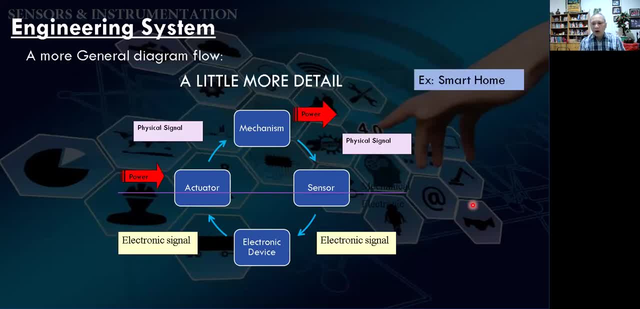 If you look at it, the home, smart home, before that, the physical quantity, which is the mechanism, is doing something and then giving power. okay, receive power and then do some activity And then, because it is making changes in physical world, then the sensor will take that and 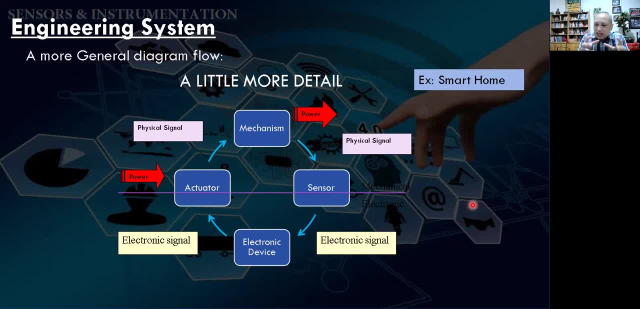 then change it to electrical signal using electronic device for the control, And then when it is having a decision what to do, then it will send signal to the actuators. can be motors, for example. just run faster, run slower and then do some more mechanism. 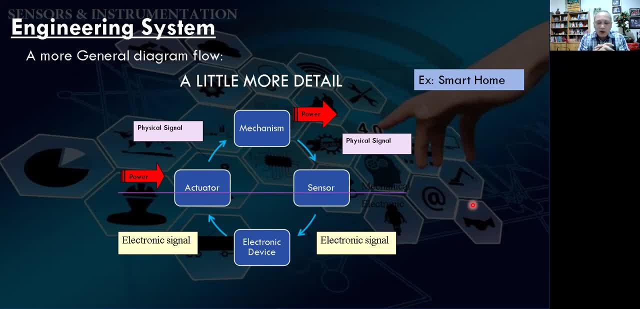 just like smart home. yeah, Just like smart home in terms of opening your gate, in terms of turning up the volume of your entertainment, music, Turning up the light, turning down dim the light, and so on and so on. So this is actually what happens there, yeah. 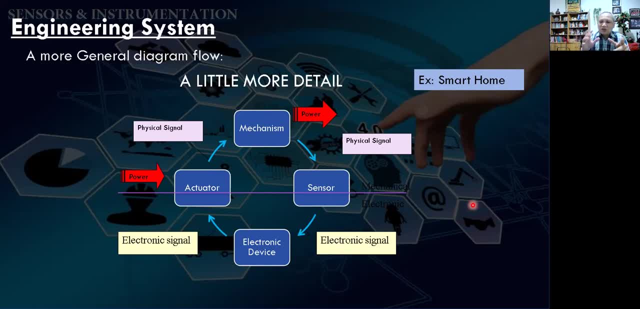 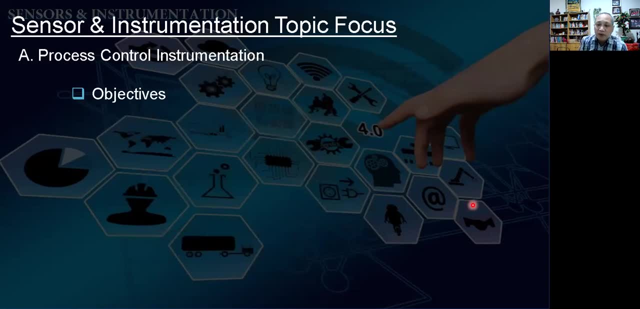 So there are sensors. actuators can be summarized into this simple four block diagrams. Okay, let's look at our topic. focus just on this course. First, of course, we will talk about process control instrumentation. yeah, We'll talk about the objectives here. 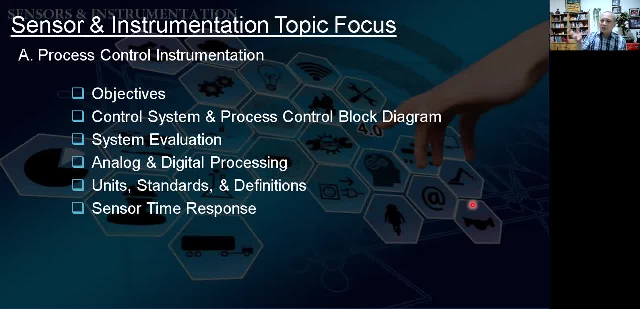 We'll talk about how, How a process control block diagram, how to evaluate the system and then how the analog and digital processes happening. Of course, we also may mention a bit about unit standards and definition, so that we can go on with full understanding what we are talking about. 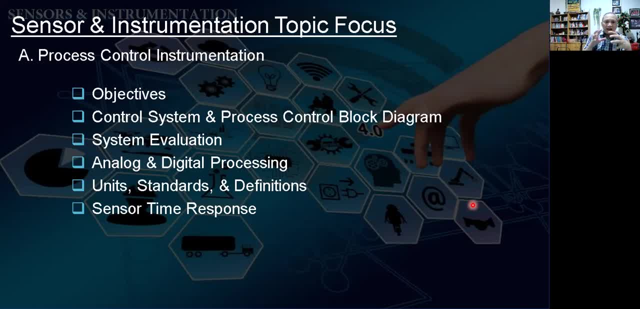 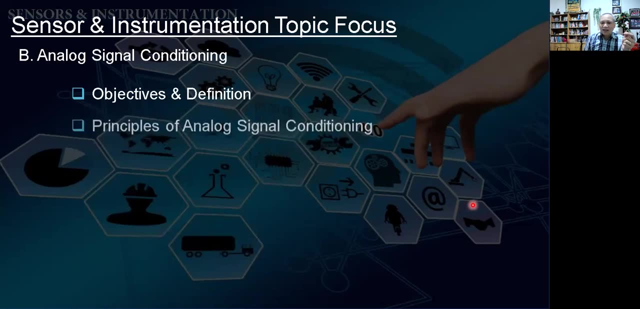 And then, of course, there is a sensor time response. This is in the part we call as process control instrumentation, And then, of course, significance and statistics. Part B is also talking about signal conditioning, analog. yeah So the principle of analog signal conditioning, talking about passive circuits, which contains 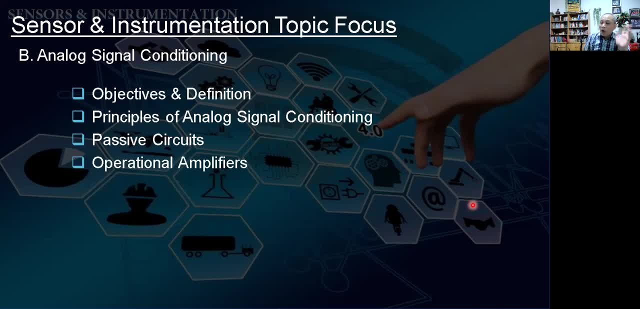 resistor capacitors and the circuits, simple circuits, op-amps. we'll talk about op-amps and then op-amps within the instrumentation. you know, op-amps we use to magnify a signal so that we can process it further. yeah, 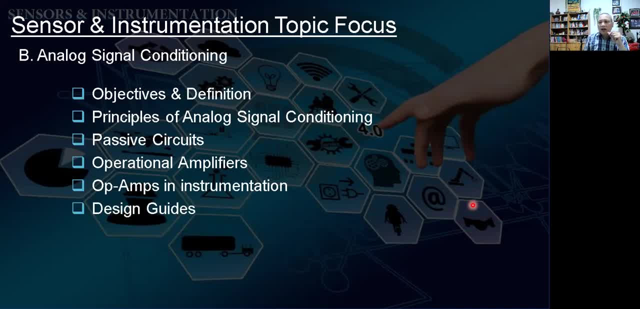 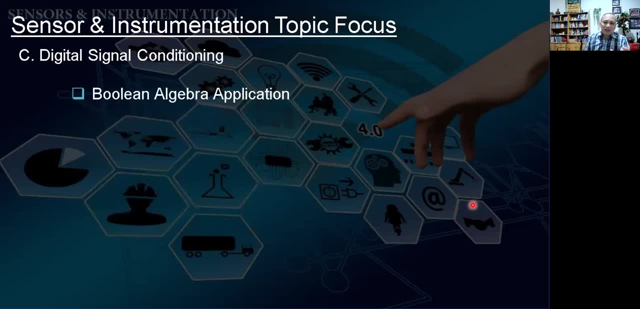 And then what is the goal? It's the guide of the design. Later we'll have a good examples of practices. yeah, See, And it was before analog and now digital signal conditioning. So we're talking about the things that probably we studied before: discrete mathematics, Boolean.